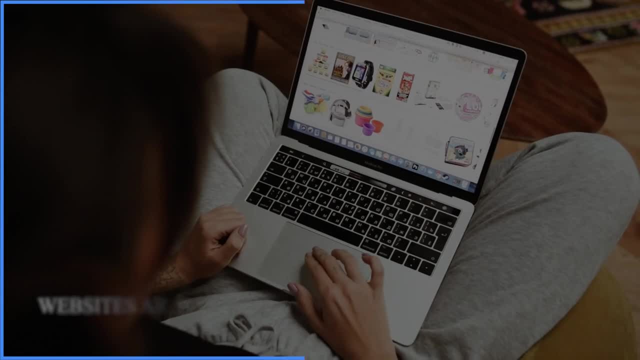 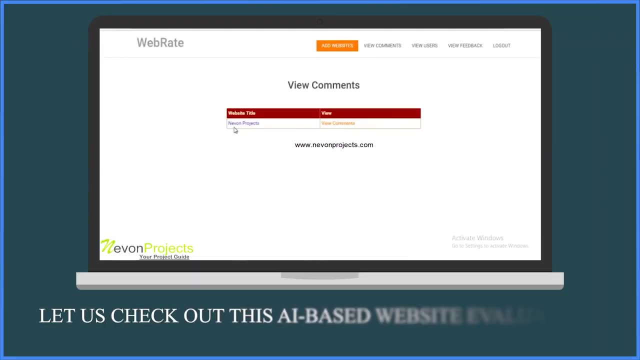 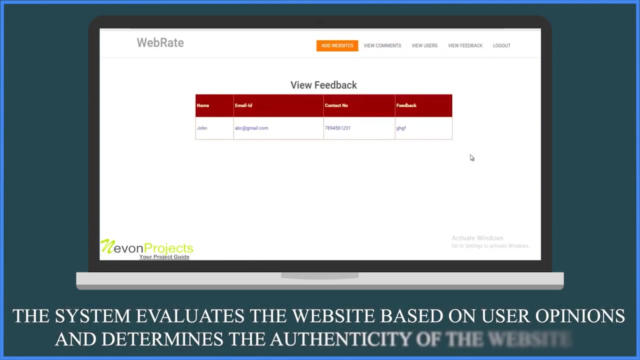 Website Evaluation using Opinion Mining. Websites are evaluated on the basis of accuracy, authority, objectivity and coverage. Let us check out this AI-based website evaluation system using Opinion Mining. This system evaluates the website based on user opinions and determines the authenticity of the website. 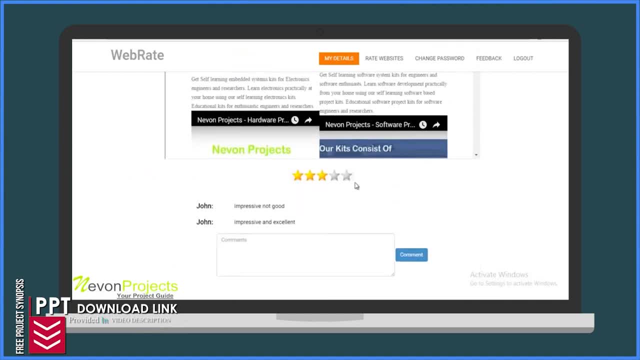 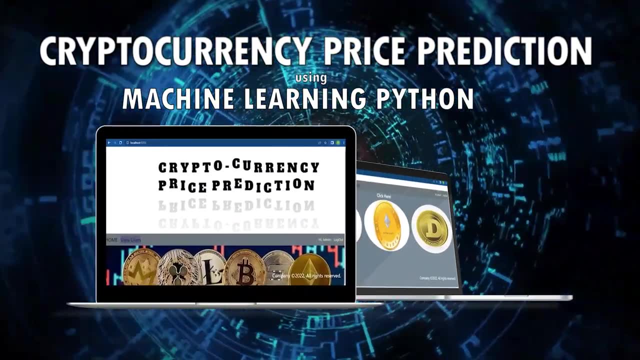 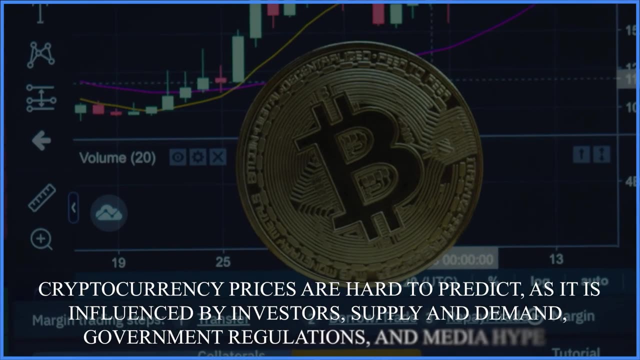 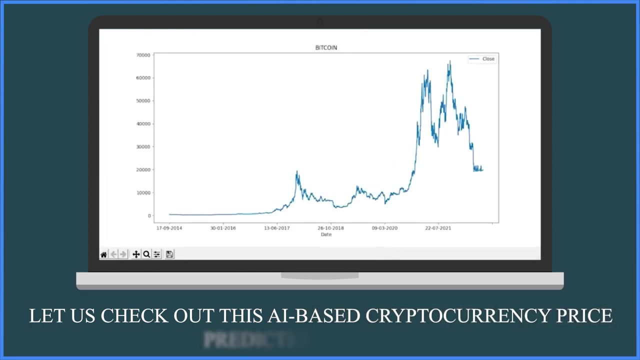 Let us check out this AI-based parle Cryptocurrency Price Prediction using Machine Learning, Python. Cryptocurrency prices are hard to predict as it is influenced by investors, supply and demand, government regulations and media hype. Let us check out this AI-based cryptocurrency prediction system. 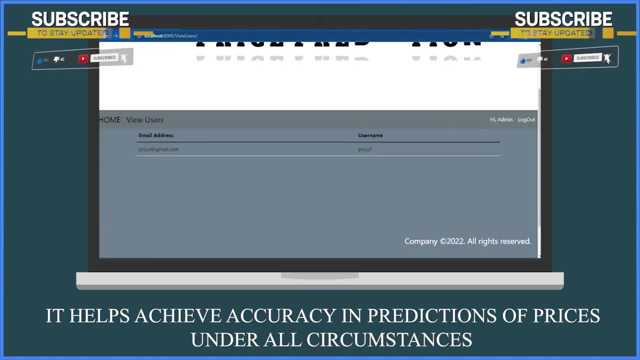 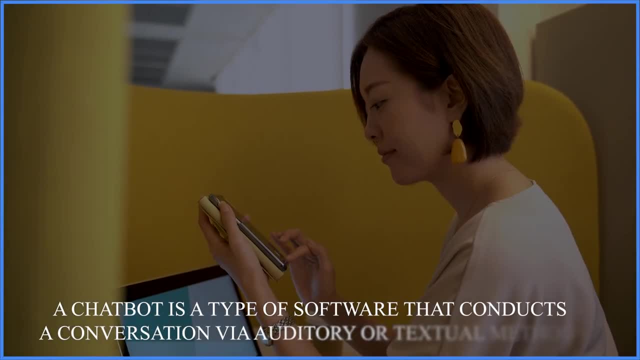 It helps achieve accuracy in predictions of prices under all circumstances. Let us check out this AI-based cryptocurrency price prediction system services under all circumstances: Online Logistics Chatbot System. A chatbot is a type of software that conducts a conversation via auditory or textual methods. 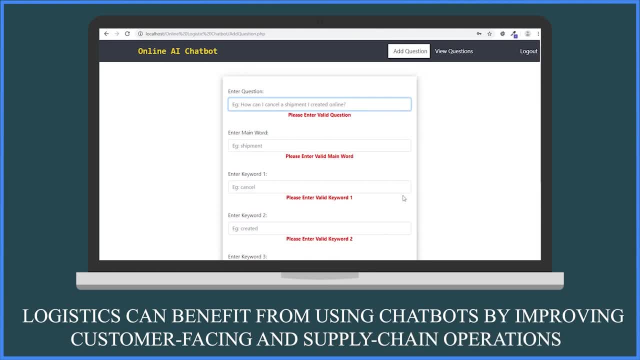 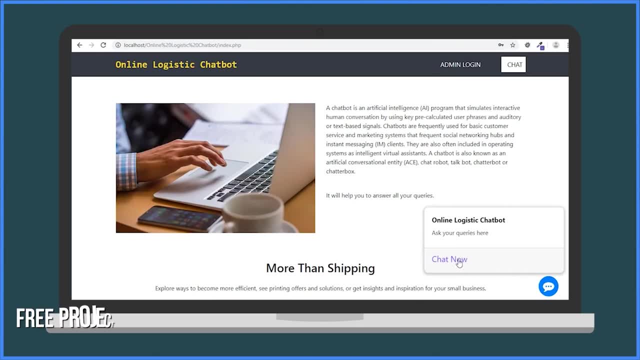 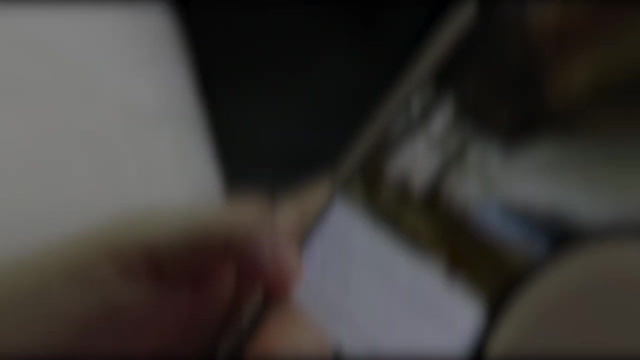 Logistics can benefit from using chatbots by improving customer-facing and supply chain operations. Let us check out this AI-based online logistic chatbot system: Quitted Trend Analysis using Latent Direct Lead Allocation. Social media users give rise to social trends as they share common interests, which can 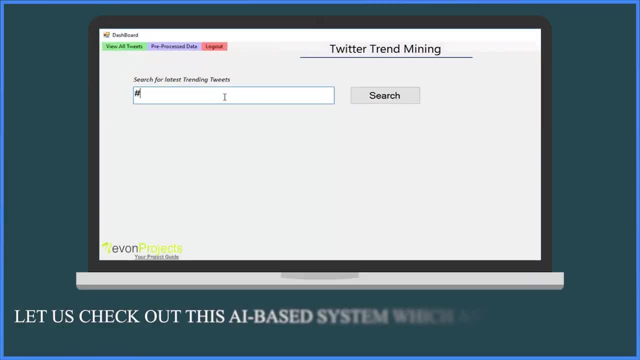 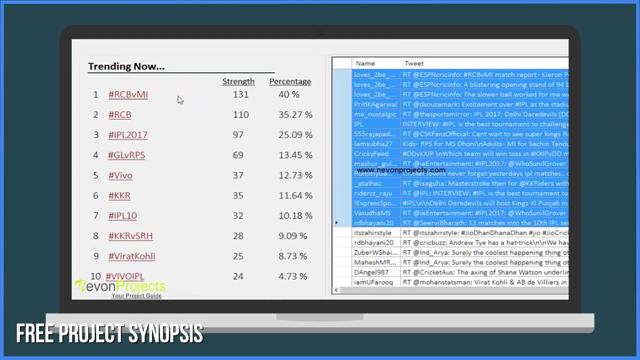 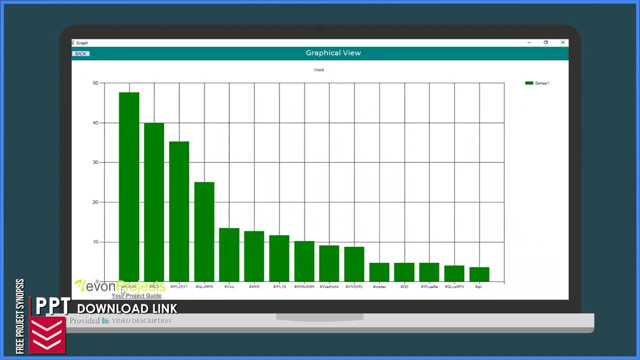 be triggered by different reasons. Let us check out this AI-based system which analyzes feedback. Let us check out this AI-based system which analyzes feedback. It can target Twitter trends based on keywords and multiple other factors. Personality Prediction System through CV Analysis. 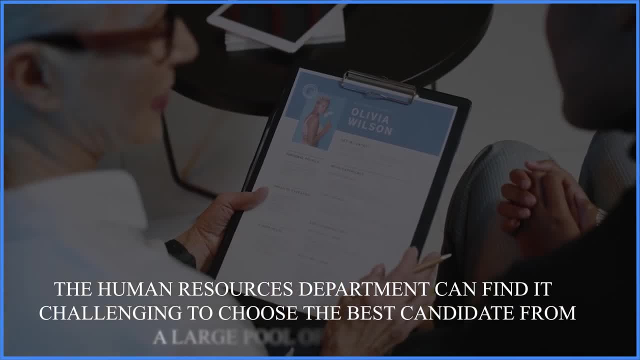 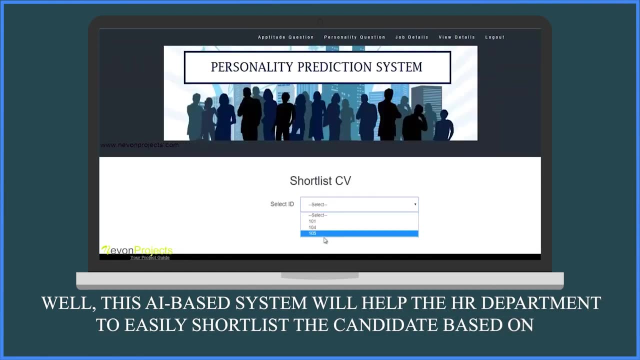 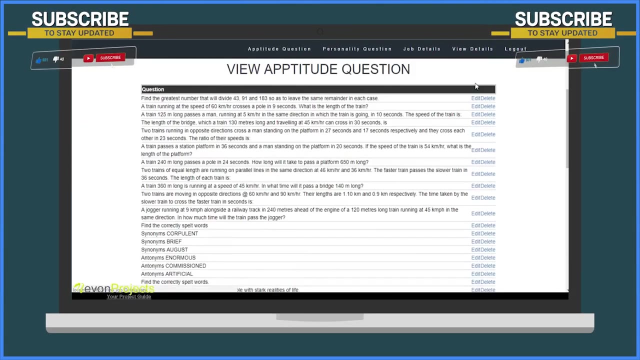 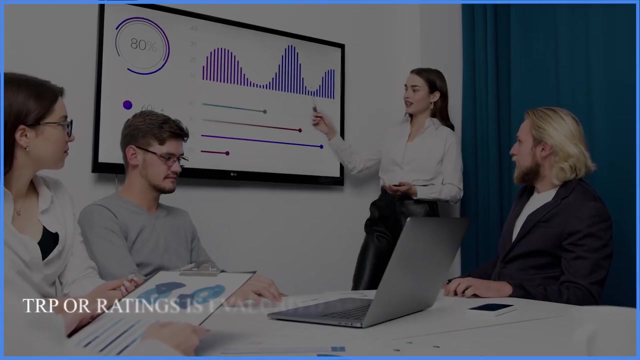 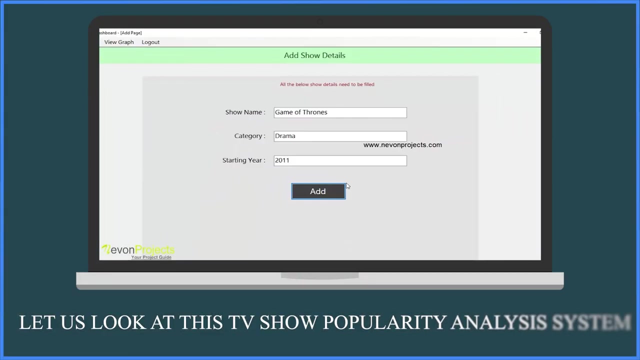 The Human Resources department can find it challenging to choose the best candidate from a large pool of applicants. Well, this AI-based system will help the HR department to easily shortlist the candidates based on the CV ranking policy, Validation of Fundamentals and Results. TV Show Popularity Analysis using Data Mining.